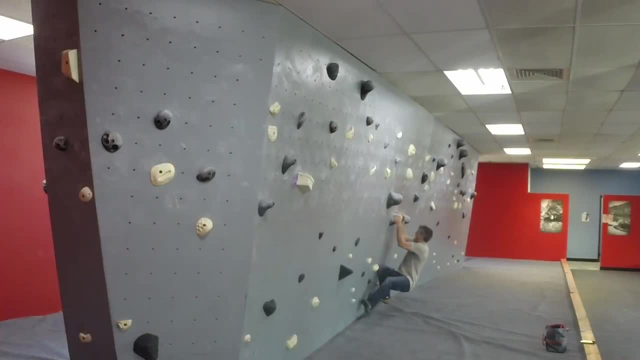 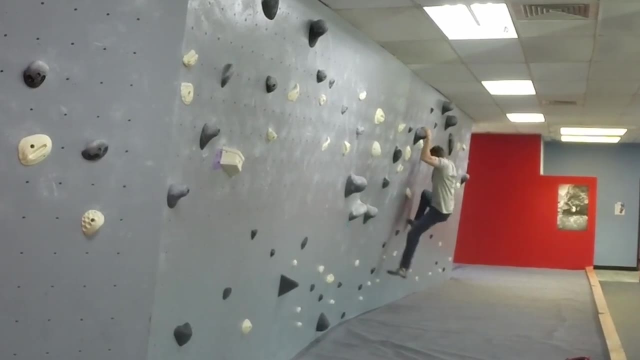 forth. I found the medium to be pretty difficult in itself and I can imagine if you wanted to do multiple laps on this would be very tough and very endurance and you're going to be really good and efficient about your shakeouts and things like that. 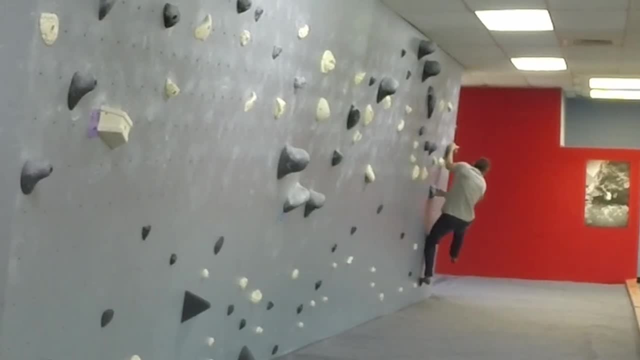 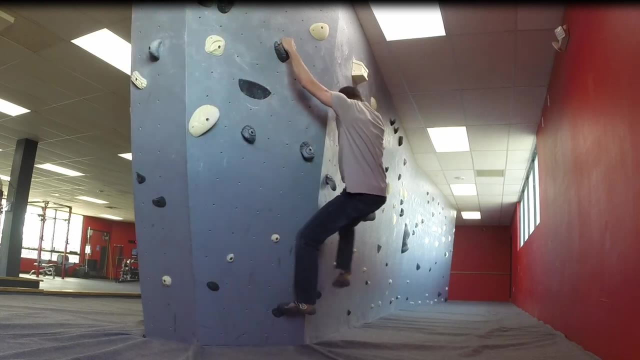 This is an abundance of different approaches and there's just a general view. I would say that really helps you guys make your own best decisions about how you want to go about your 위에 and crossings, So it's pretty easy. I've been doing this for the past eight years and I can't believe. 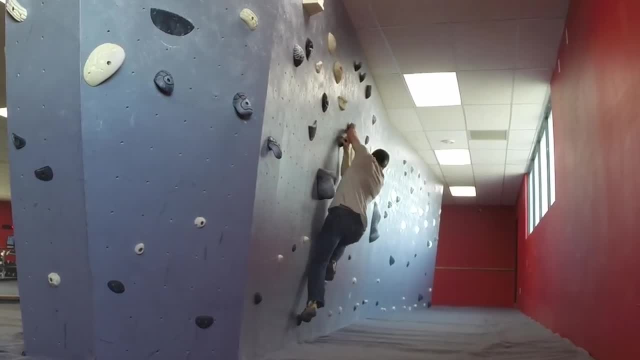 it's just not working. It's pretty normal. So this is just basically a variety of different íais And I think that I will show you guys some of the things that I do. So this is my little video And I'm probably going to show you guys the cannabisIT basics. 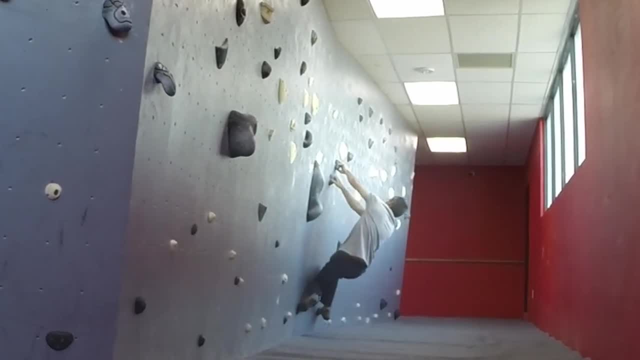 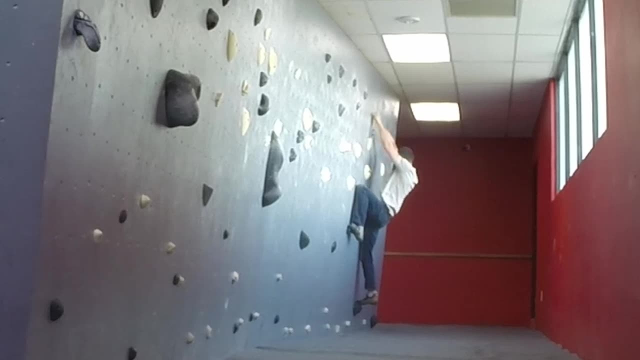 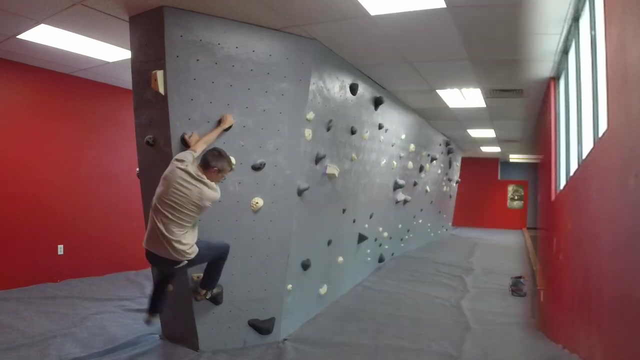 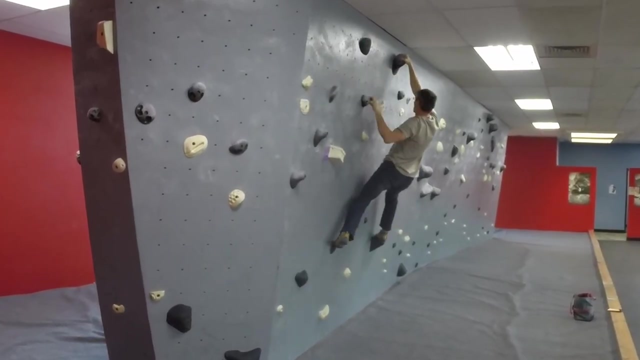 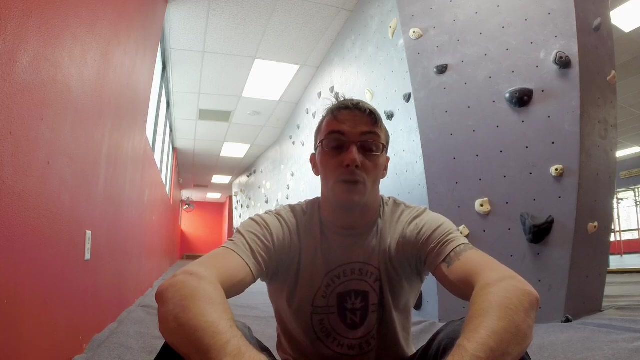 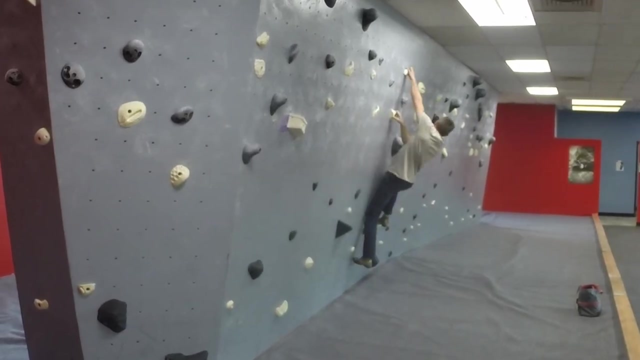 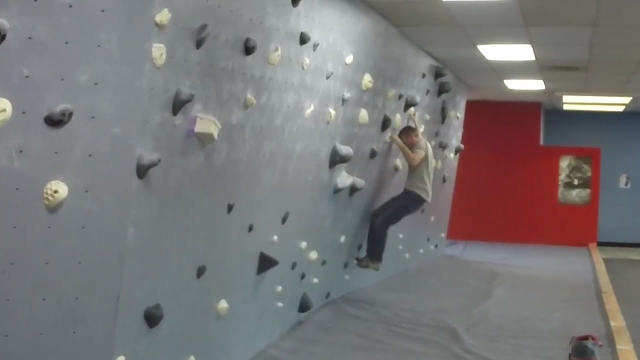 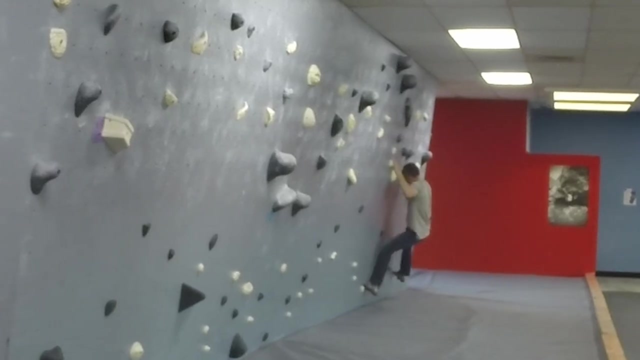 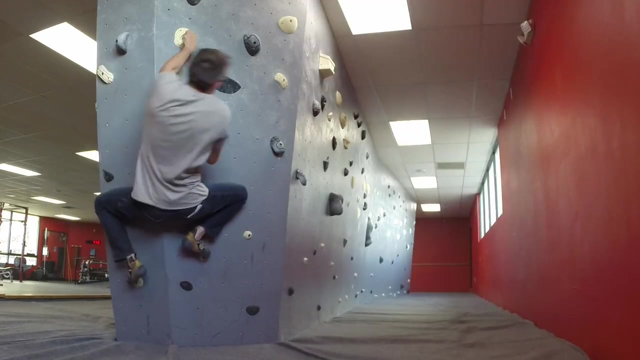 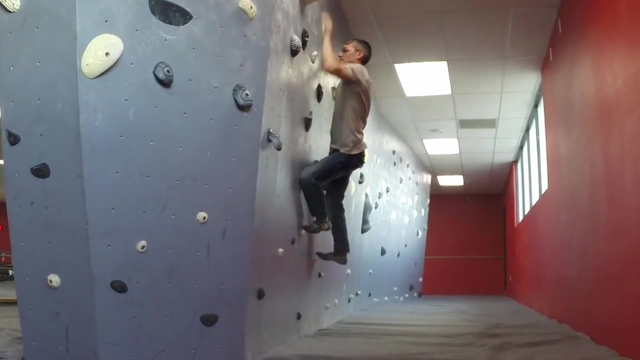 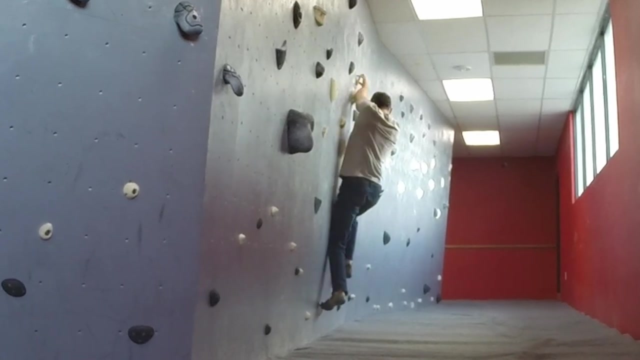 a little bit. So the cannabisIT basics. So with the cannabisIT basics you're going to see the barreles at the top and the white was quite tough. you- i actually didn't even make it all the way around on that back wall- it got quite crimpy. 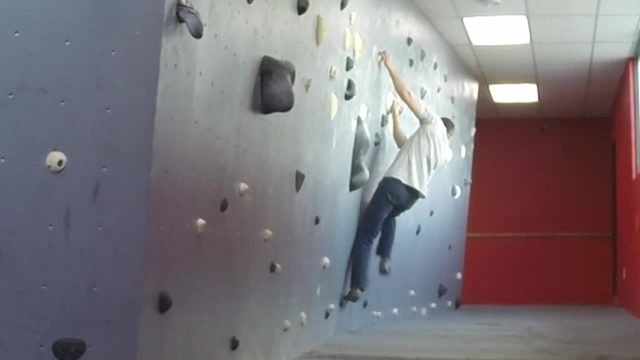 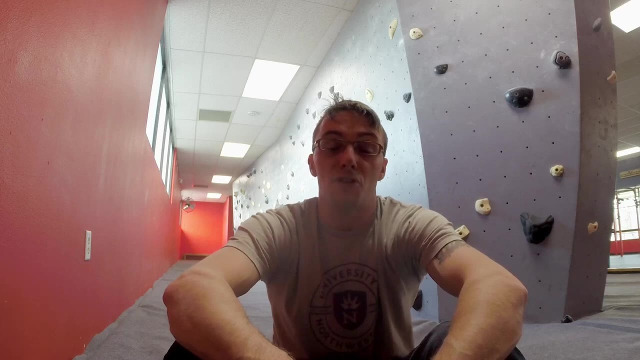 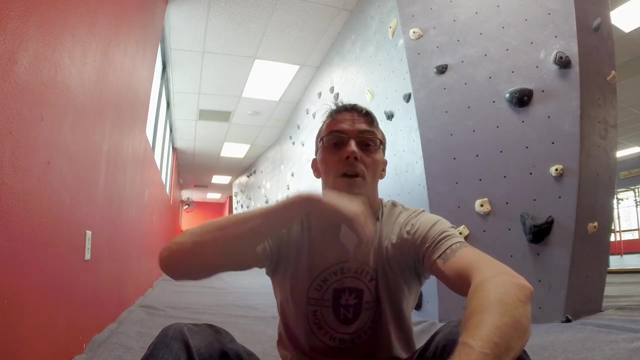 and i hadn't wired it yet, so like i didn't, probably wasn't using the best technique, but definitely feeling the forearm pump here on my home wall. at home i have the endurance weave. uses pretty nice comfy jugs and it's a up and down and around and then reverse up and down. 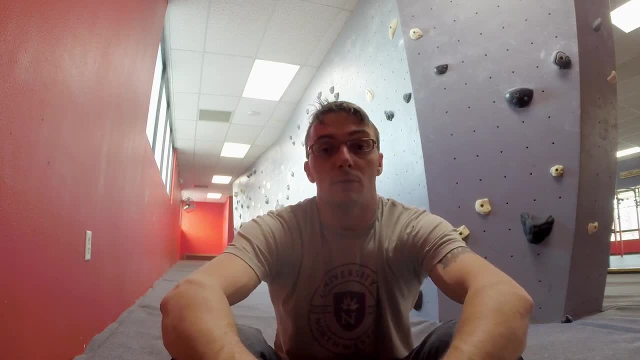 and around my home wall and outside, of just doing more and more moves, getting into the hundreds or more of moves on these bigger jugs at home, i can definitely see it getting to where i need to make the holes a little bit smaller, a little bit more difficult. this style of thing here is pretty.